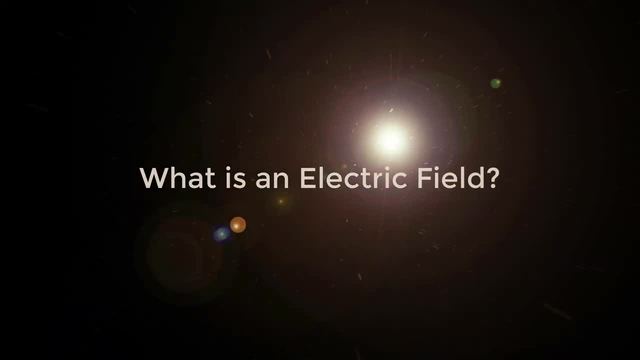 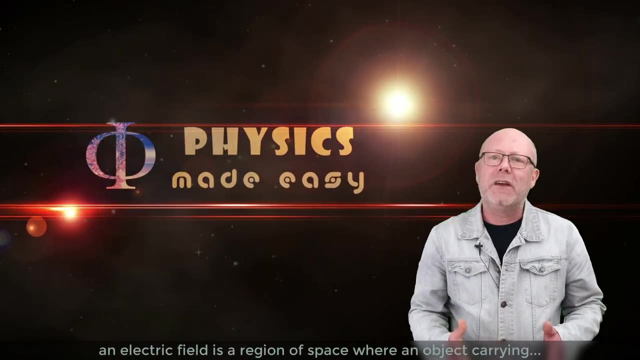 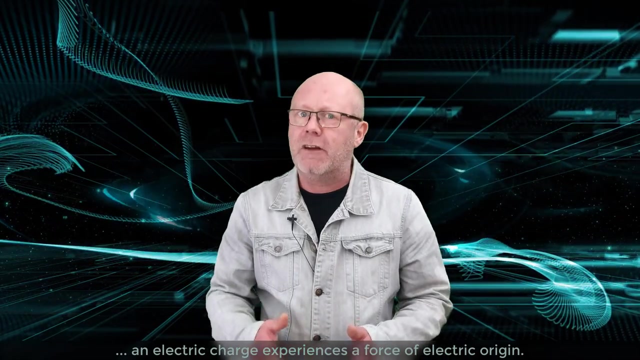 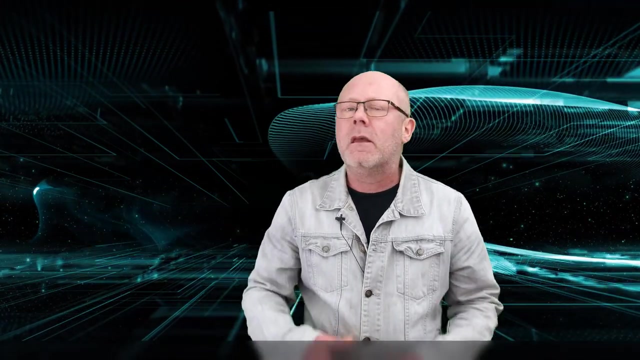 What is an electric field? In a nutshell, an electric field is a region of space where an object carrying an electric charge experiences a force of electric origin. Let's look at this definition in order to understand all of its facets. In electric field there's a word field. 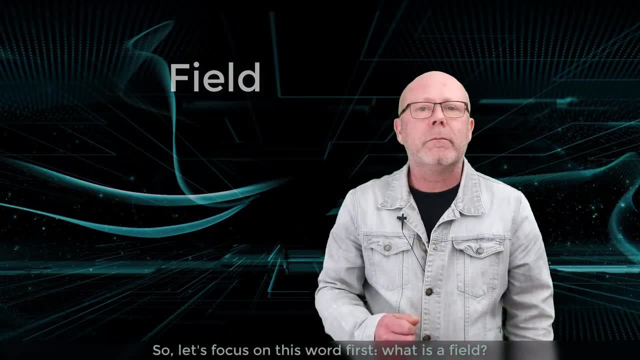 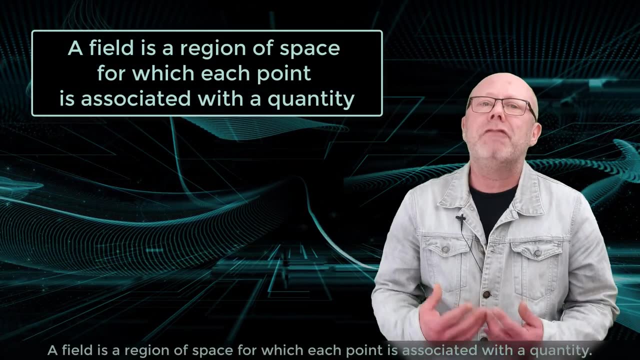 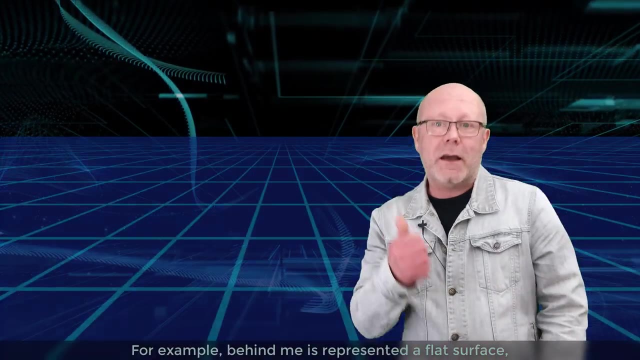 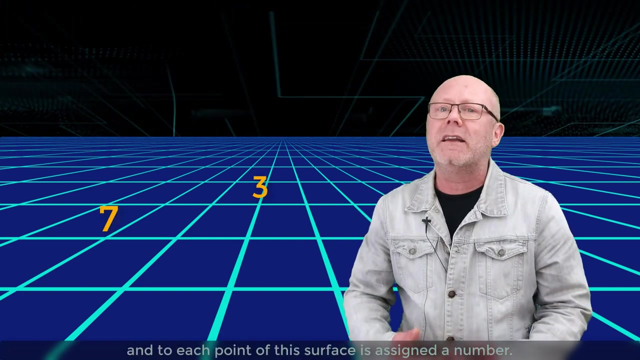 So let's focus on this word first. What is a field? A field is a region of space for which each point is associated with a quantity. For example, behind me is represented a flat surface and to each point of this surface is assigned a number, The property associated with that. 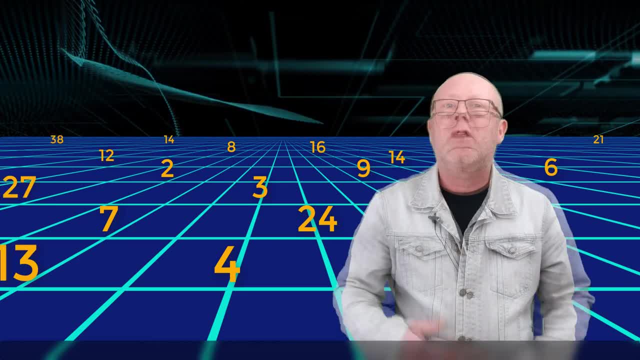 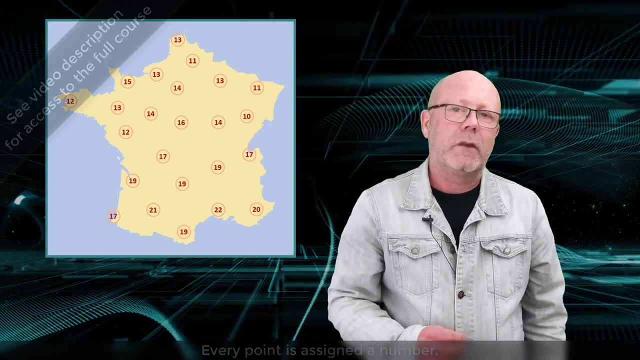 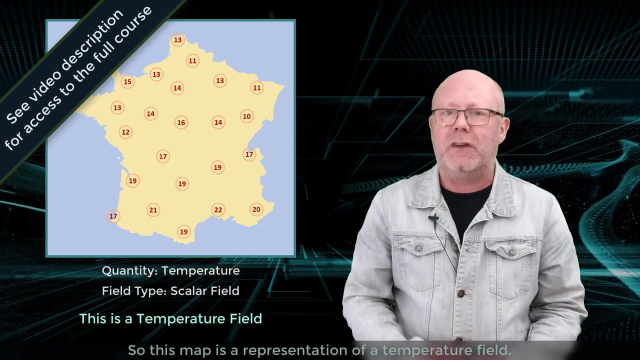 quantity defines the nature of the field. To understand what this means, let's look at this map. Every point is assigned with a number. This number represents the temperature of the point. So this map is a representation of a temperature field. You can try this with other type of 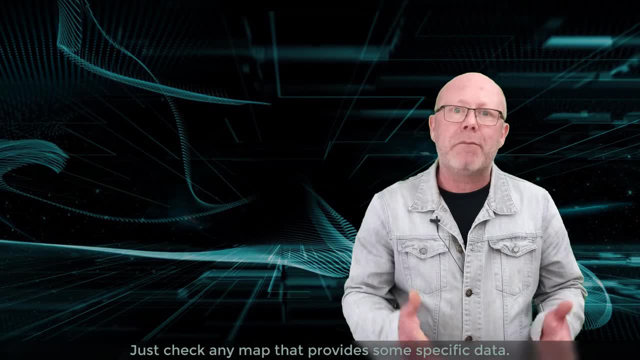 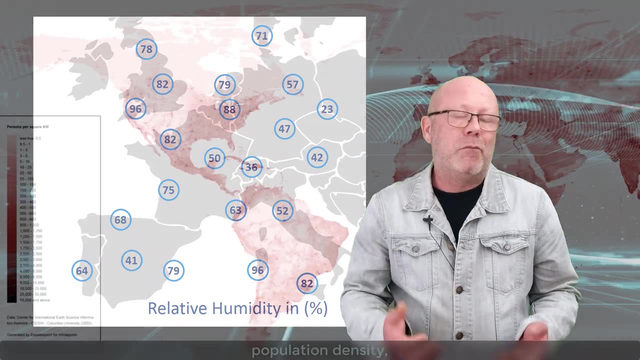 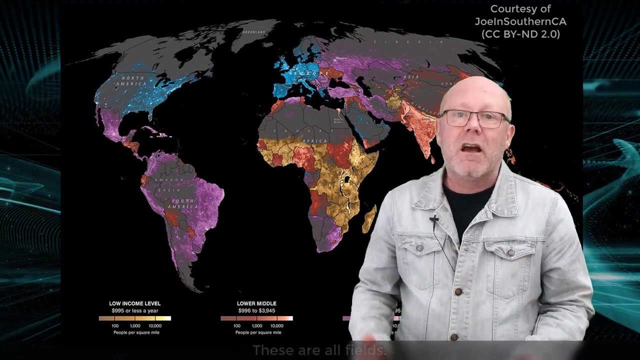 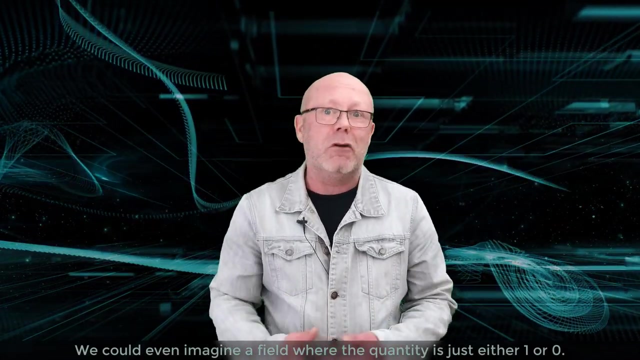 quantities. Just check any map that provides some specific data, like, for example, humidity, Population density or population average income. whatever These are all fields, We could even imagine a field where the quantity is just either 1 or 0. For example, an electron field. Yes, imagine. 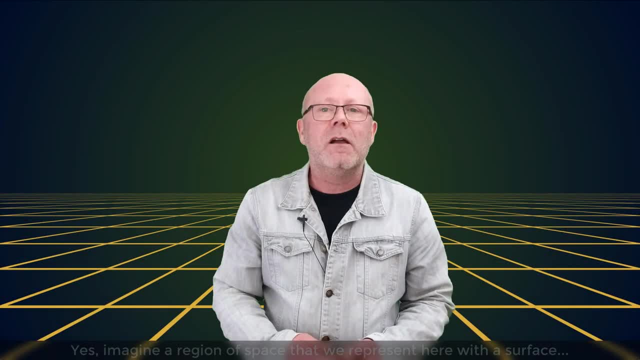 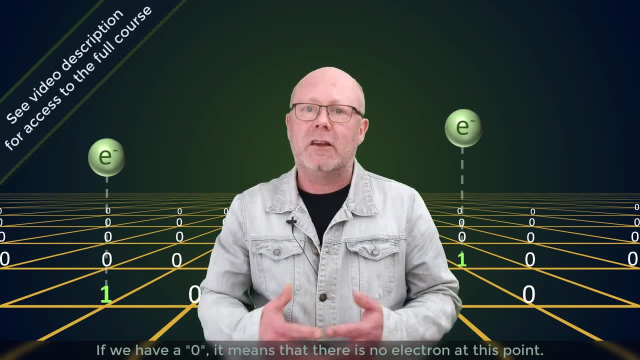 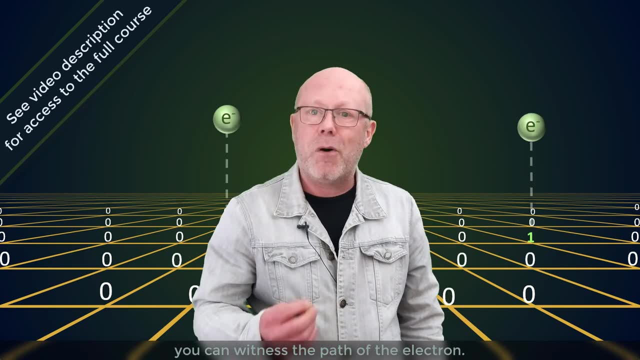 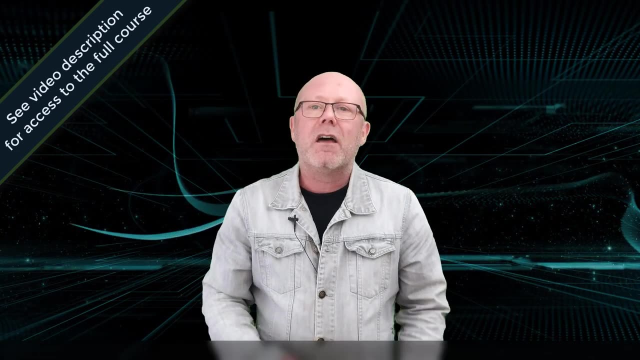 If we have a 0, that means there is no electron at this point. If you look at the evolution of the field with time, you can witness the path of the electron. We can also imagine that, instead of a number, the quantity associated with each point is a vector. 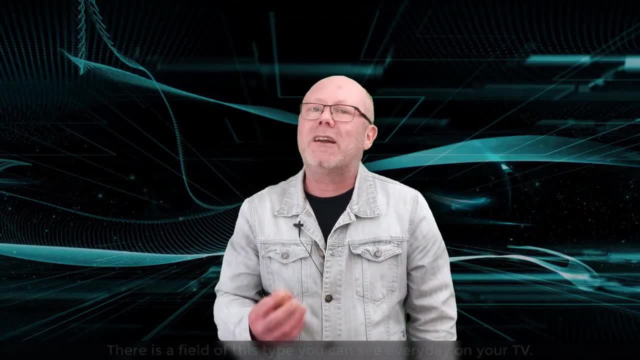 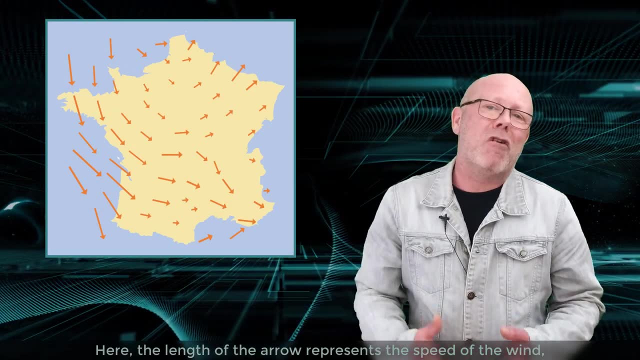 which is a value with a direction. There is a field of this type, you, that you see every day on your TV. This one Here, the magnitude of the arrow represents the speed of the wind and the direction of the arrow, the direction of the wind. 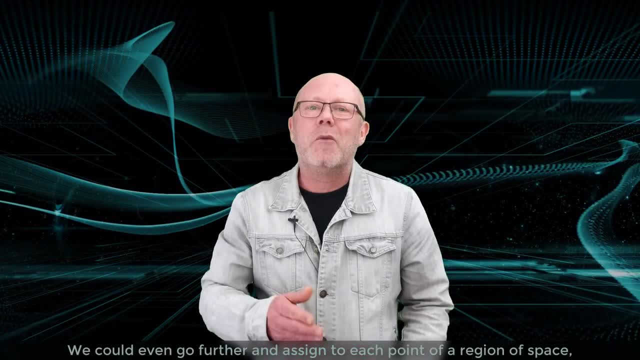 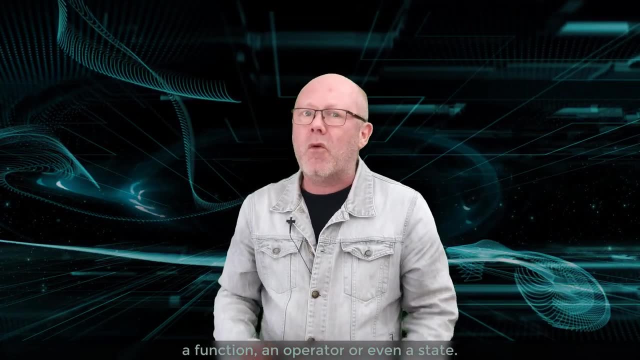 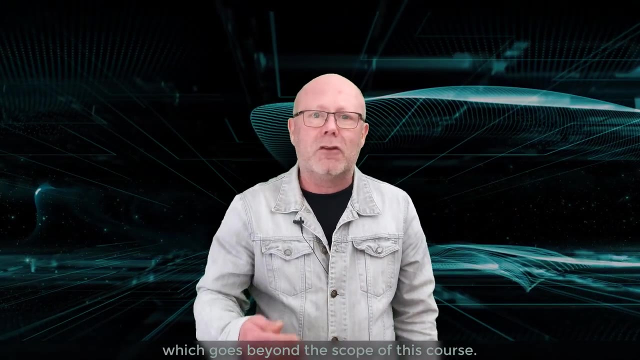 That field is our vector field. We could even go further and assign to each point of a region of space a function, an operator or even a state. But looking into this would make us dive deep into quantum field theory, which goes beyond the scope of this course. 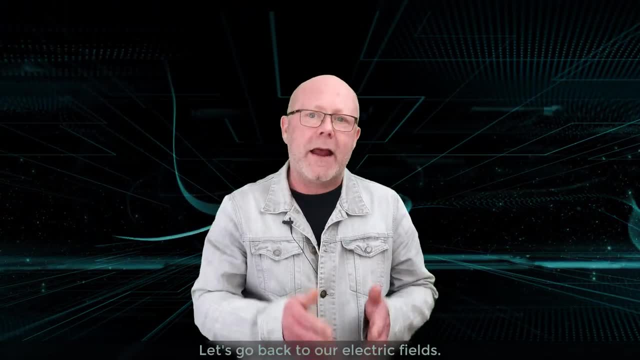 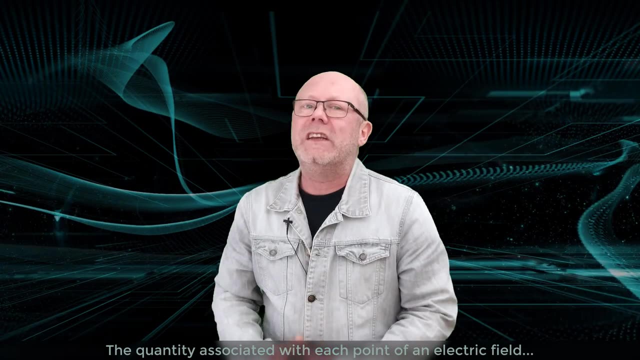 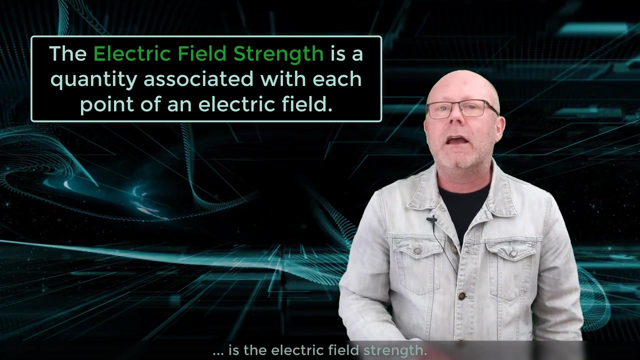 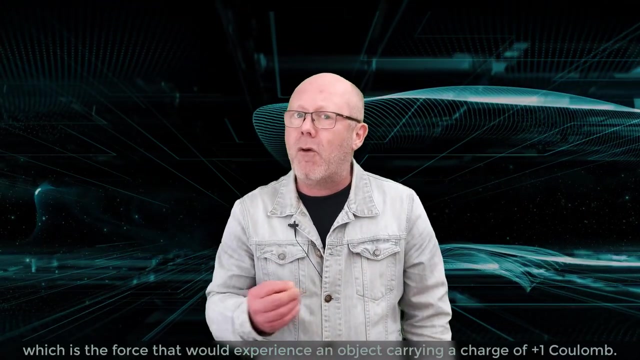 So let's go back to our electric fields. The quantity associated with each point of an electric field is the electric field strength. As its name suggests, this quantity represents the strength of the effect of the field, which is the force that would experience. 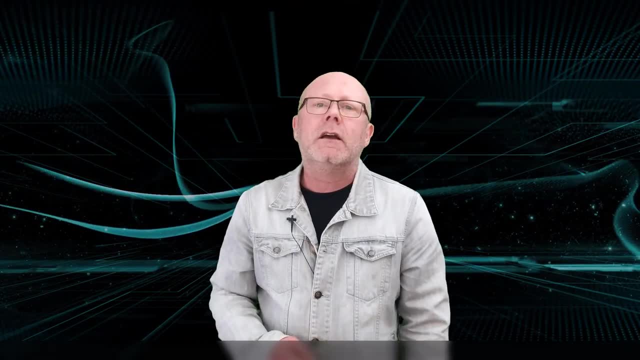 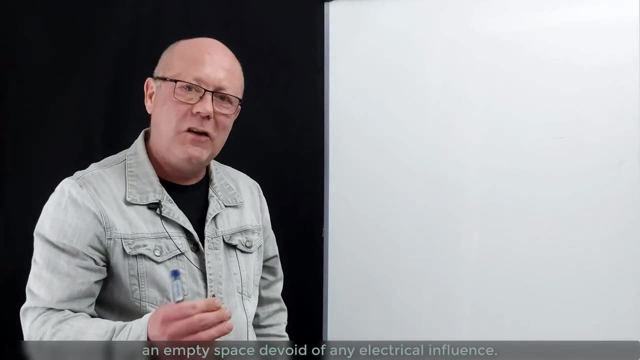 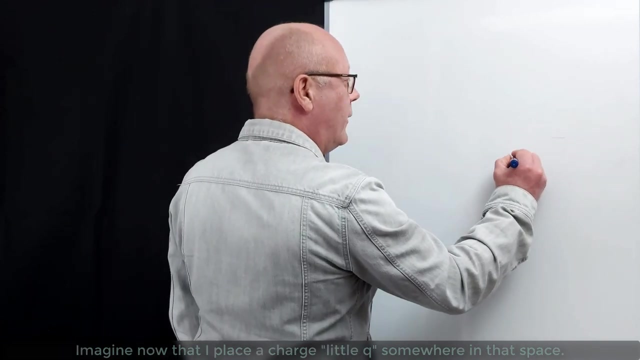 an object carrying a charge at one coulomb. Let me pull out the board to illustrate this. Imagine: this board is an empty space, An empty space devoid of any electrical influence. Imagine now that I place a charged little cube somewhere in that space. 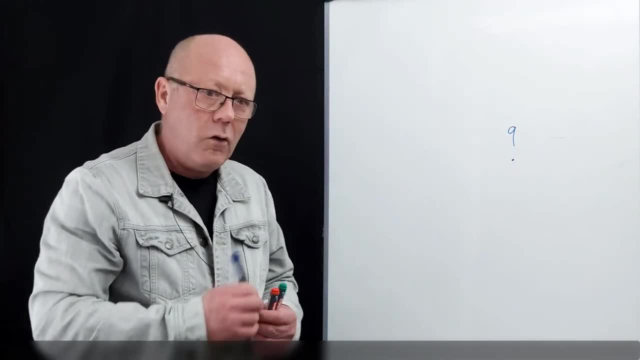 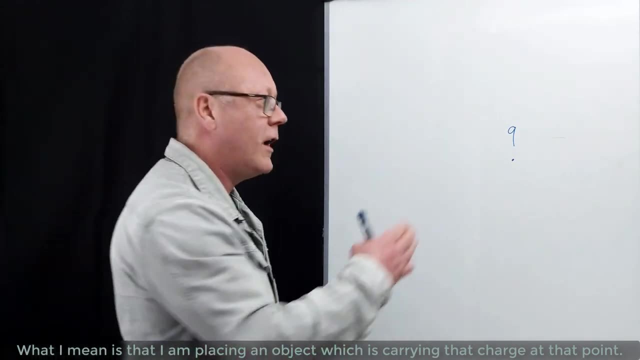 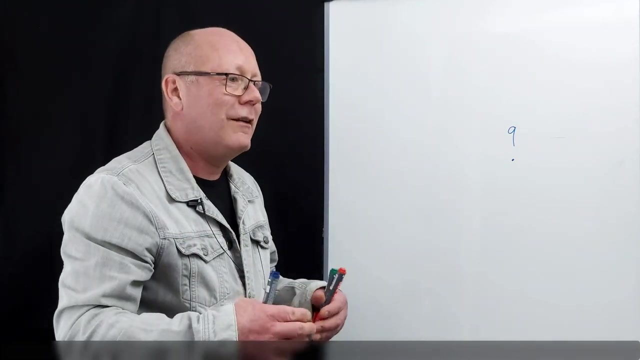 A positive charge. Oh yeah, When I say that I'm placing a charge at a given point, what I really mean is that I'm placing an object which is carrying that charge at that point. Remember, charge is a property, But in this course, 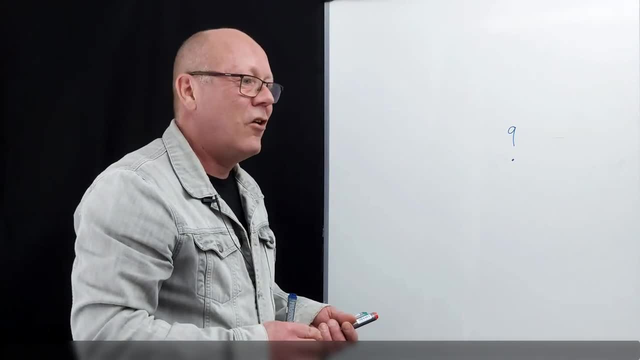 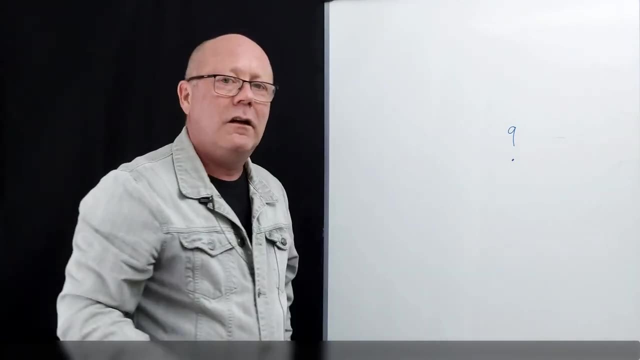 I'll be placing lots of charge a bit everywhere. So I'm not going to say each time I place an object which is carrying this charge. I'll just say I'm placing a charge. But do remember that a charge is a property, not a thing. 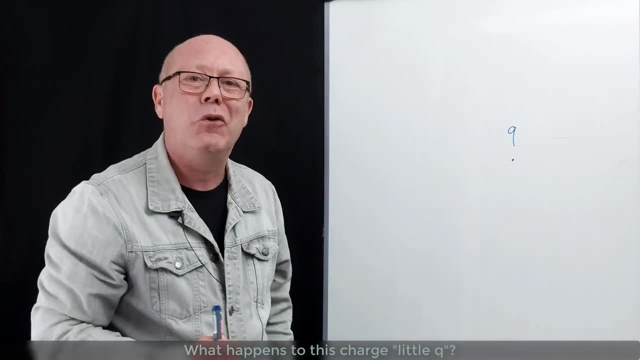 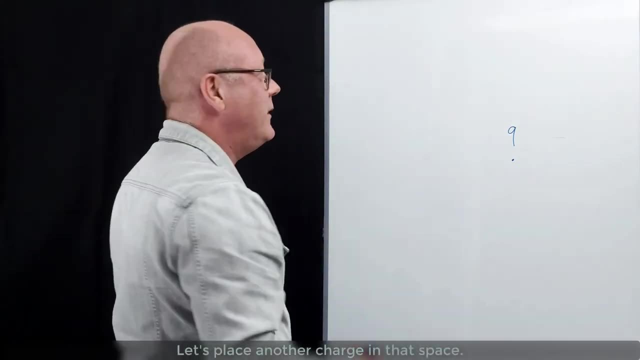 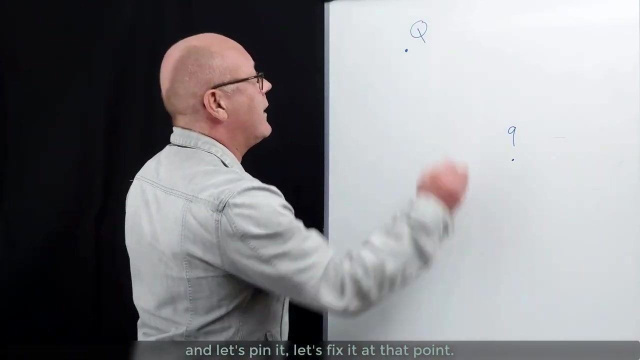 Okay. So what happens to this charged little cube? Well, nothing, Okay. So let's place another charge in that space. Charge big Q positive 2. And let's pin it. Let's fix it at that point. 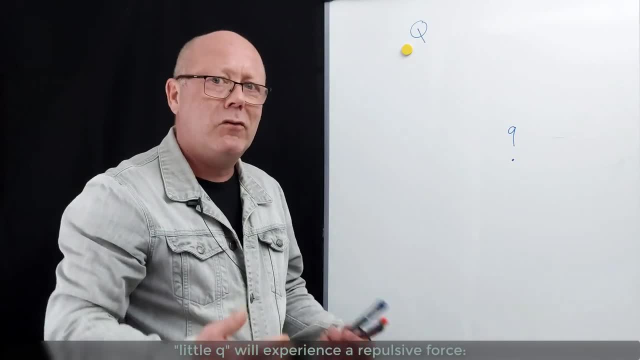 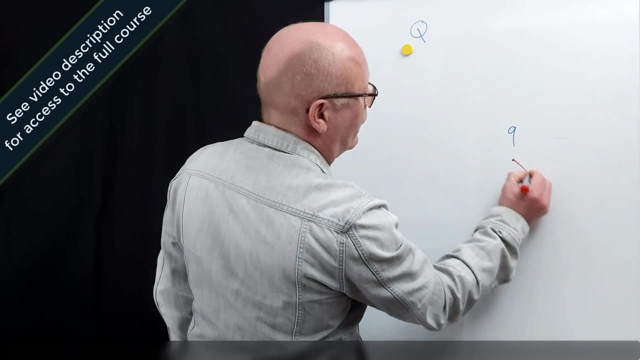 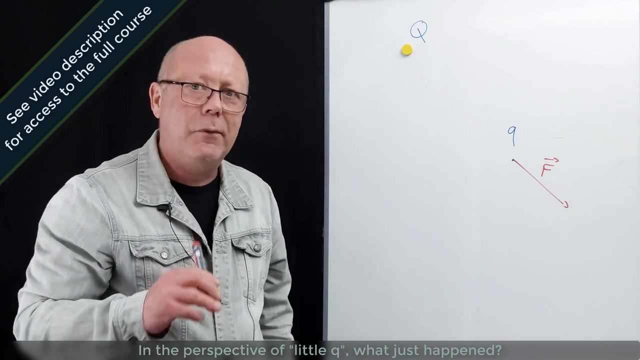 Little Q will experience a repulsion force. Yeah, Positive and positive repel. So there'll be a force on little Q. In the perspective of little Q, what just happened? It was just there not doing much right. Suddenly it feels accelerated. 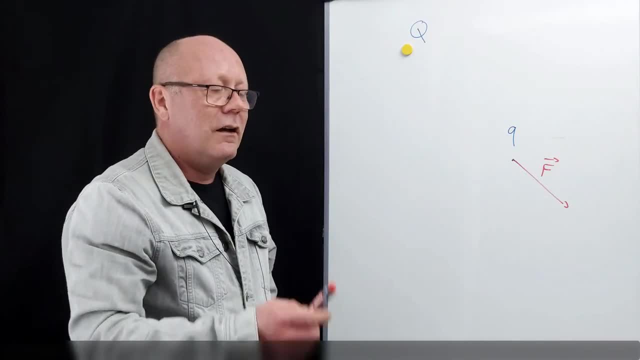 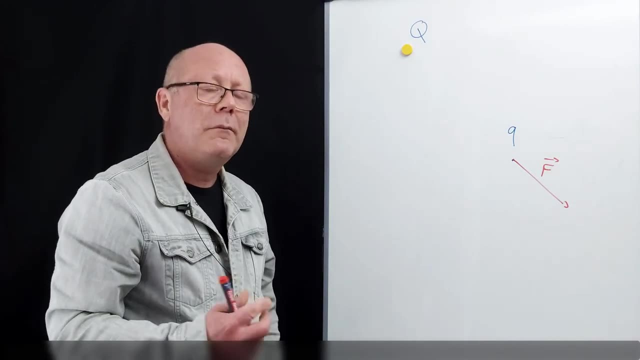 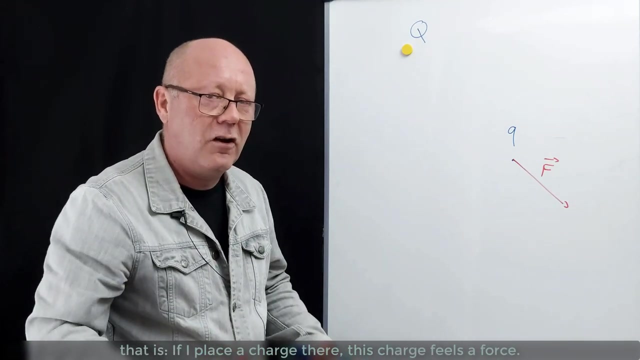 There's a force applied on it In its perspective. something changed fundamentally in the nature of space itself. Something new happened. Now the point where it was located has a new property, That is, if I place a charge there, this charge feels a force. 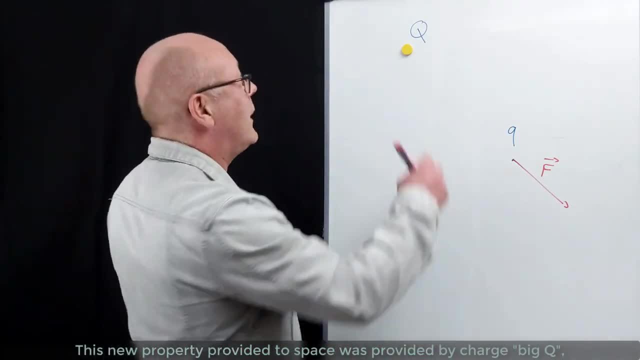 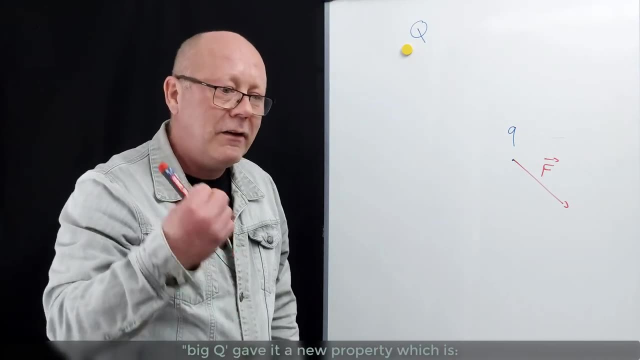 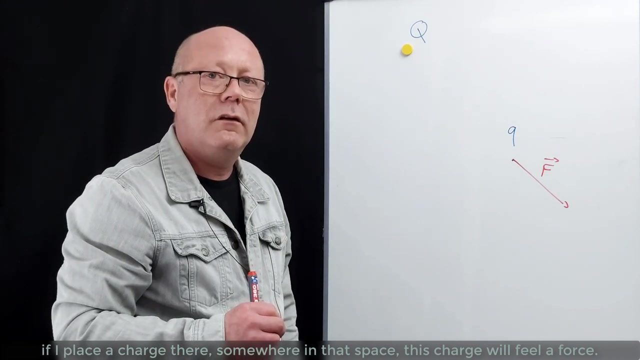 This new property provided to space was provided by charge, big Q- That actually modified the region of space around it. It gave it a new property, which is: if I place a charge there somewhere in that space, this charge will feel a force. 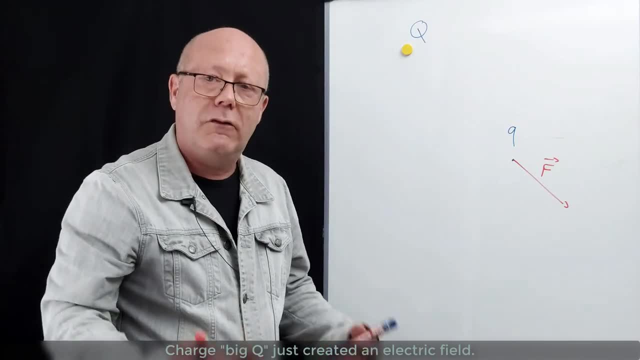 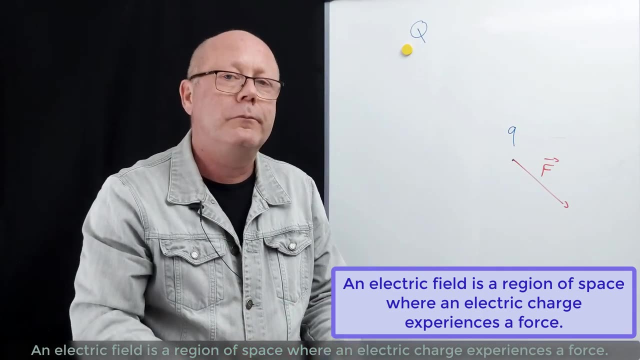 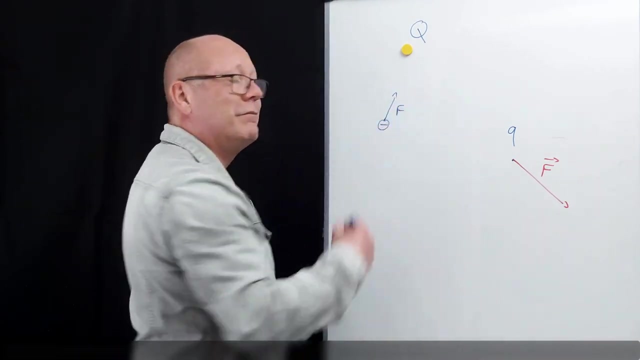 Charge. big Q just created an electric field. An electric field is a region of space where a charge experiences a force. So if I placed a charge here- for example a negative 1, it would feel a force. A positive 1. 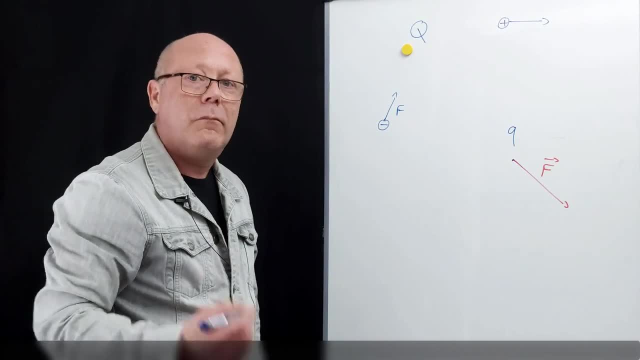 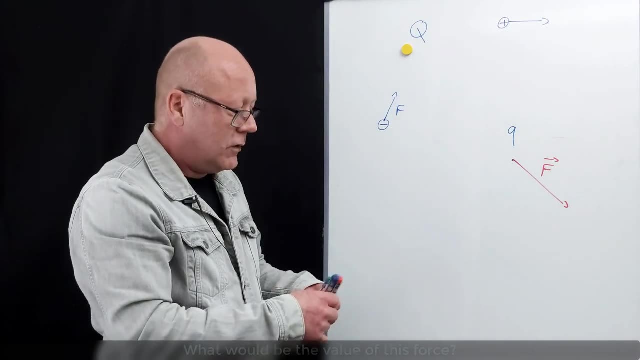 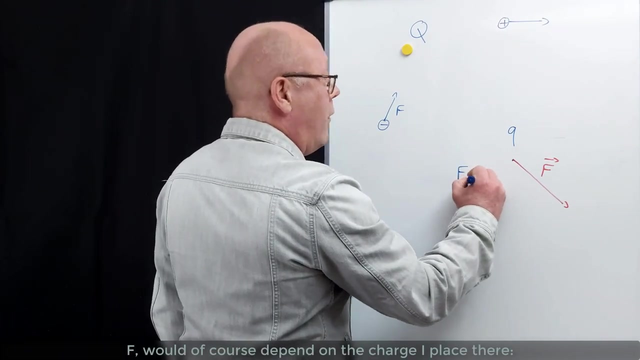 here would feel a force Because it is in the electric field, created by charge. big Q, Okay, So what would be the value of this force? Let's go back to our charge little q here. F would of course depend on the charge I place there. 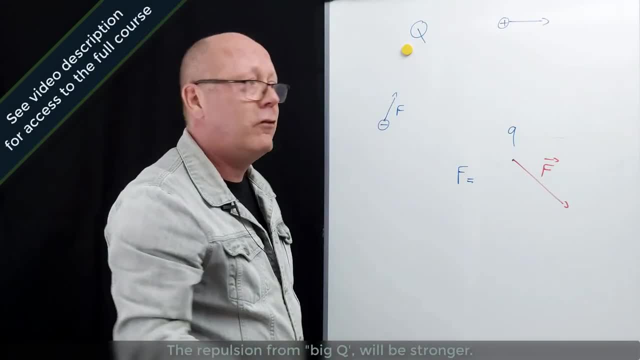 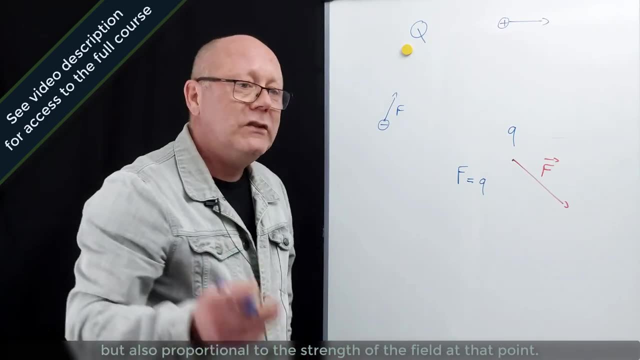 If I place a big charge, well, the force on it will be bigger. The repulsion from big Q will be bigger. So F is proportional to the force I place at the point, but also proportional to the strength of the field at that point. 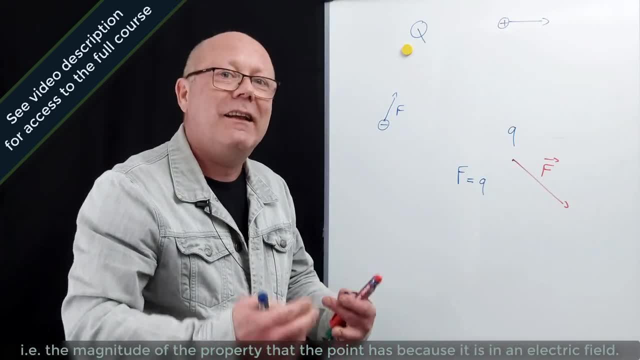 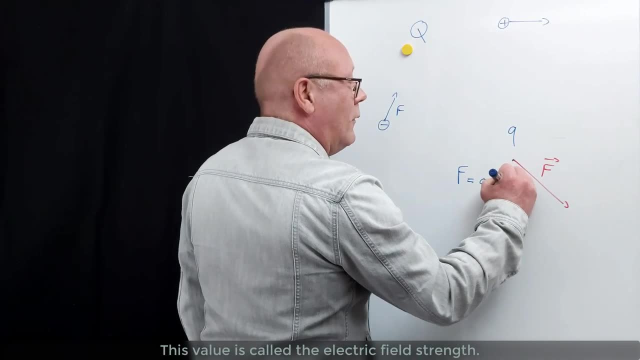 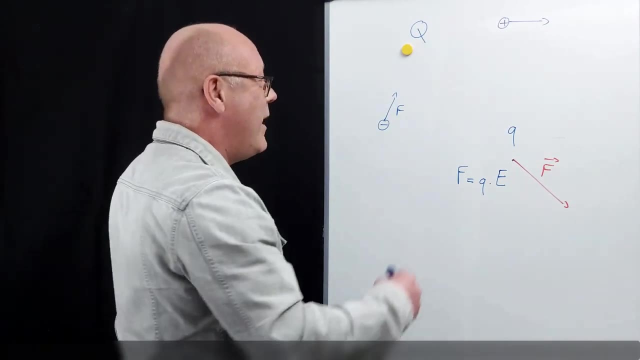 ie the magnitude of the property that the point has because it is in an electric field. This value is called the electric field strength, The strength of the field. The electric field strength is a vector, As you can see. it's proportional to a force.